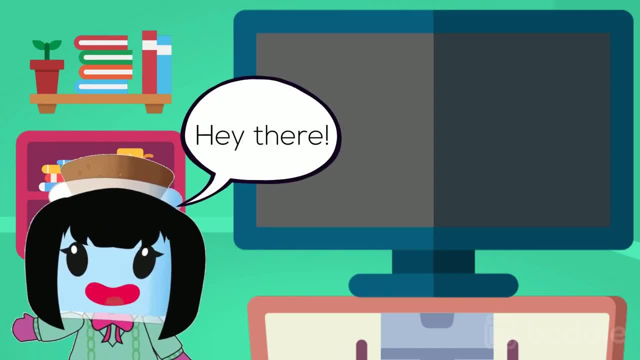 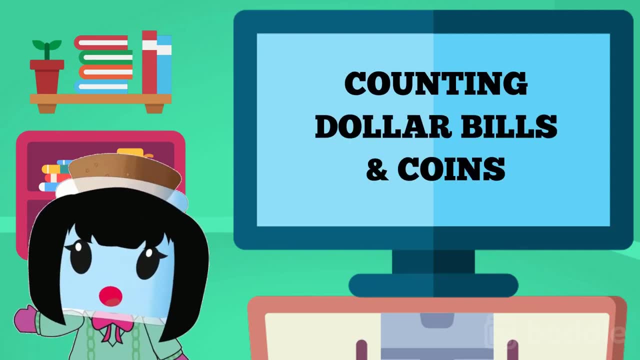 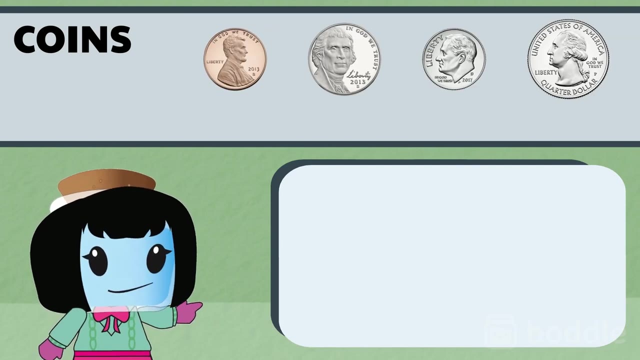 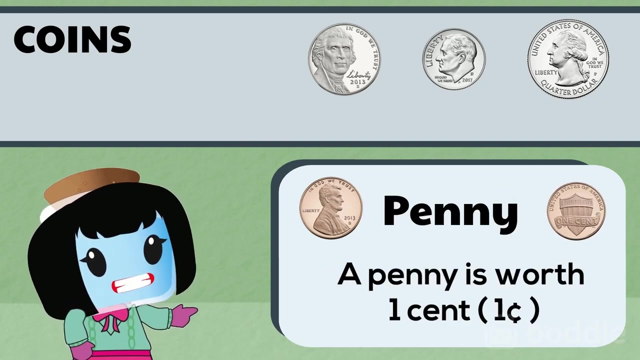 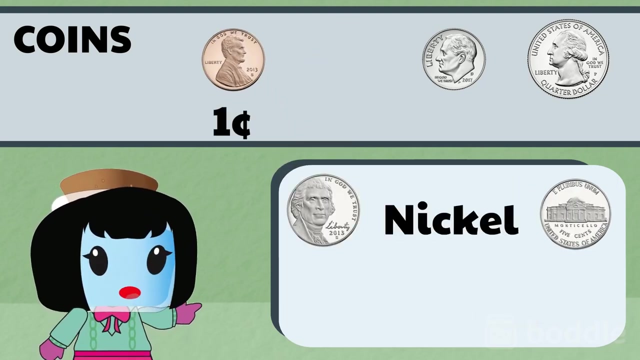 Hey there. Today we're going to learn about counting dollar bills and coins. Let's start with reviewing coins. Here we have four coins. The first one is called a penny and it is worth one cent. The second one is a nickel, which is worth five cents. The 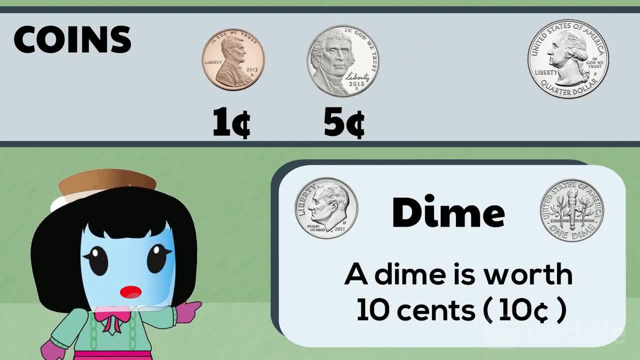 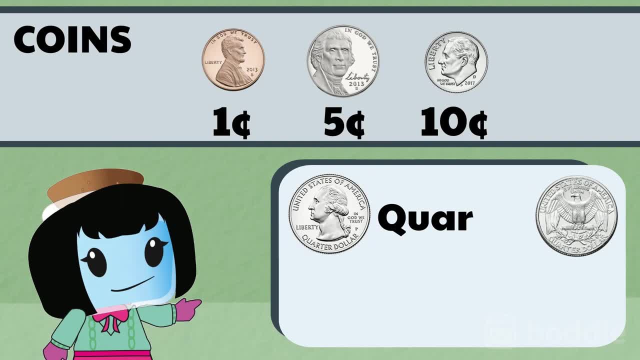 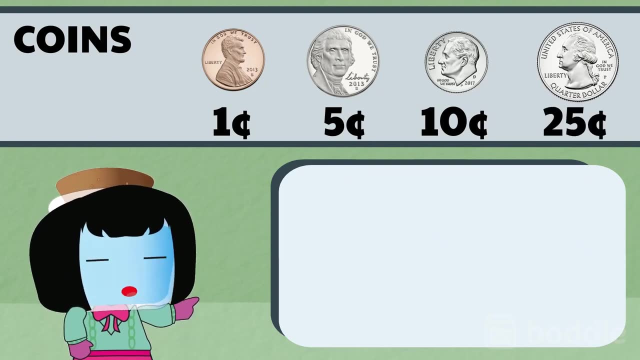 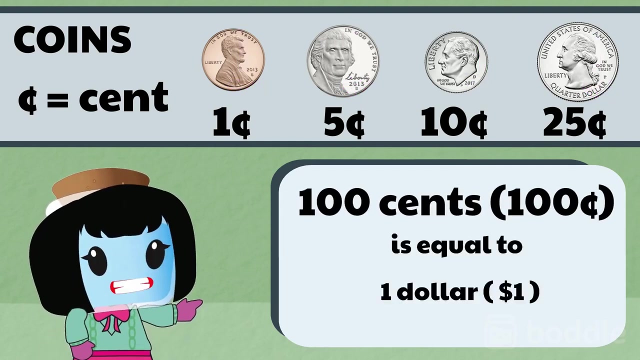 next one is a dime. It's worth ten cents. Lastly, we have a quarter, which is equal to 25 cents. As you can see, this is the symbol percent and it is placed after the number. If we have 100 cents, that's equal to one dollar Instead of a coin. 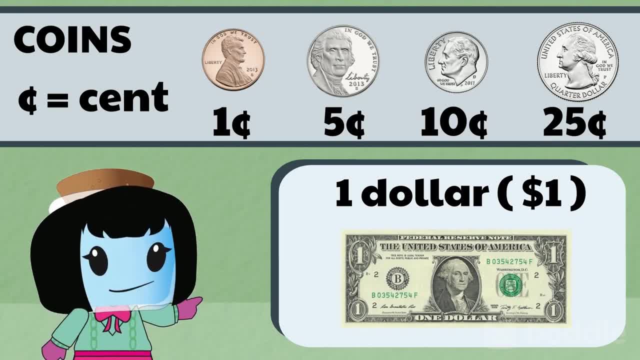 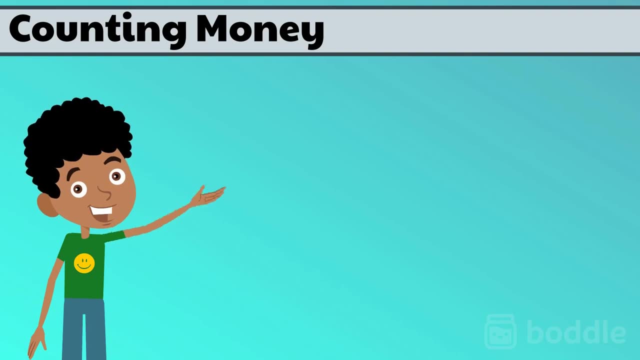 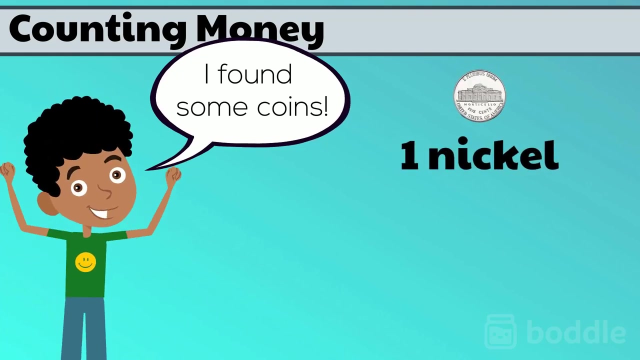 though we have a one dollar bill. Notice how this time the dollar symbol is put here Before the number. Now that we are familiar with the coins and the dollar bill, let's practice counting money by helping our friend Edward. Edward found some coins on the ground. He found one nickel and six pennies. How much did he? 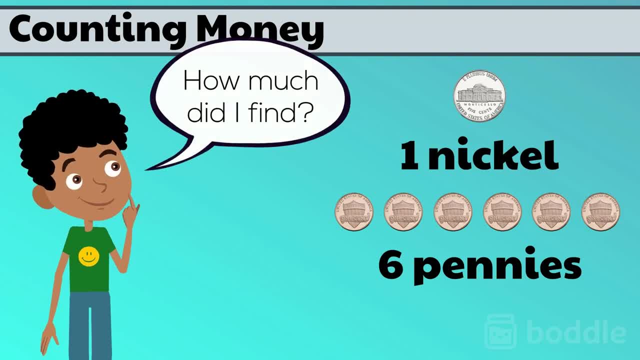 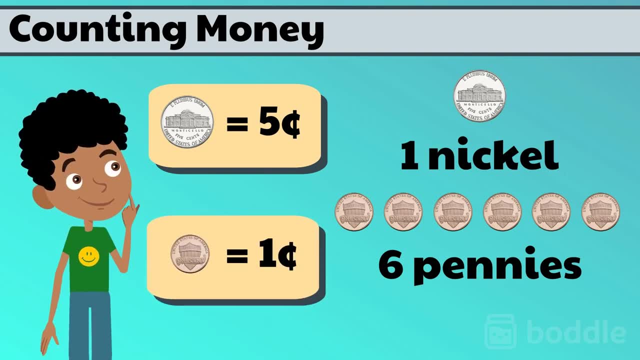 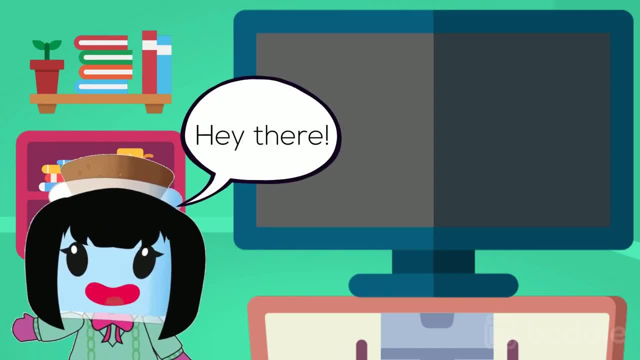 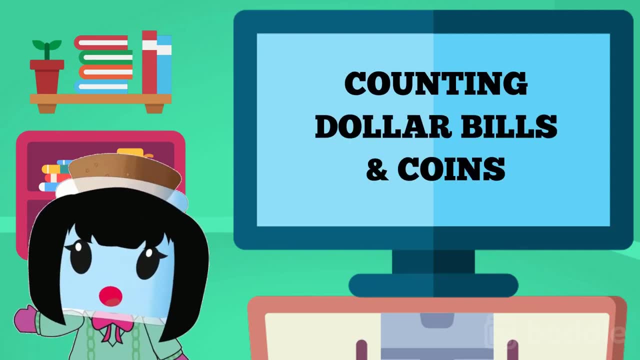 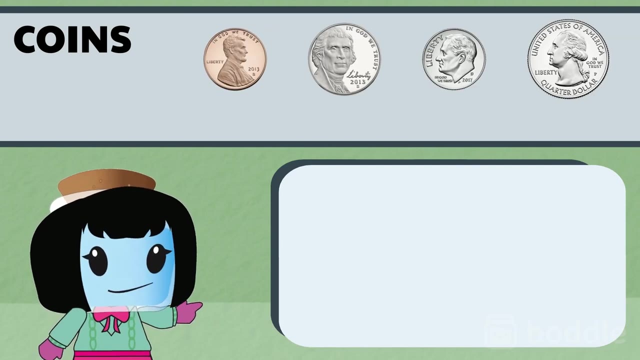 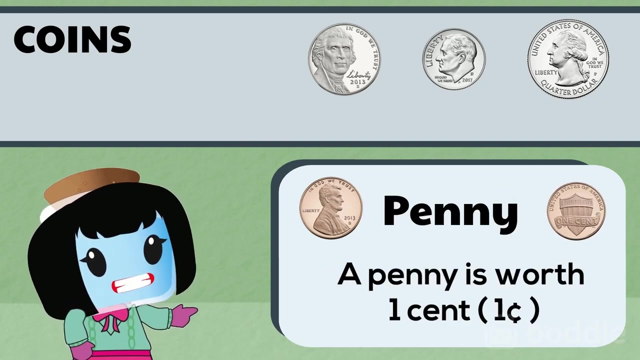 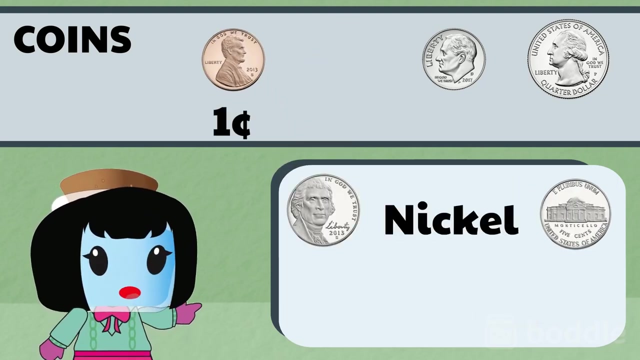 Hey there. Today we're going to learn about counting dollar bills and coins. Let's start with reviewing coins. Here we have four coins. The first one is called a penny and it is worth one cent. The second one is a nickel, which is worth five cents. The 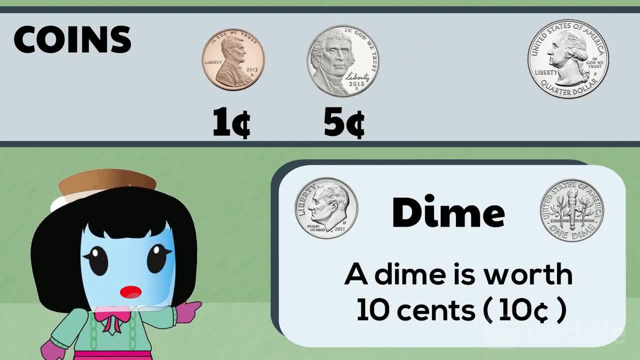 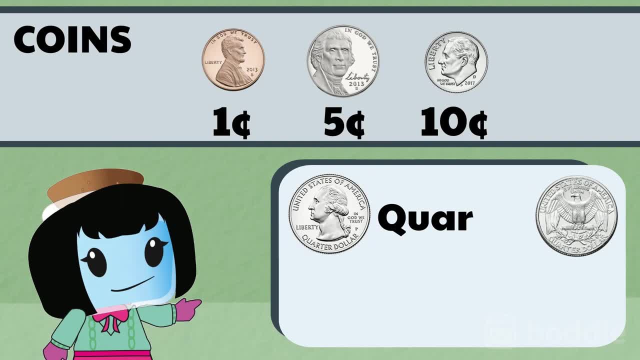 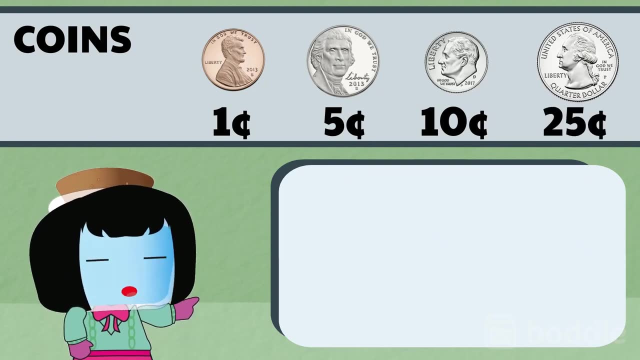 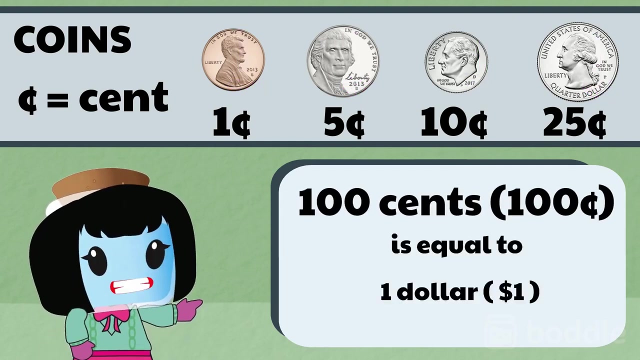 next one is a dime. It's worth ten cents. Lastly, we have a quarter, which is equal to 25 cents. As you can see, this is the symbol percent and it is placed after the number. If we have 100 cents, that's equal to one dollar Instead of a coin. 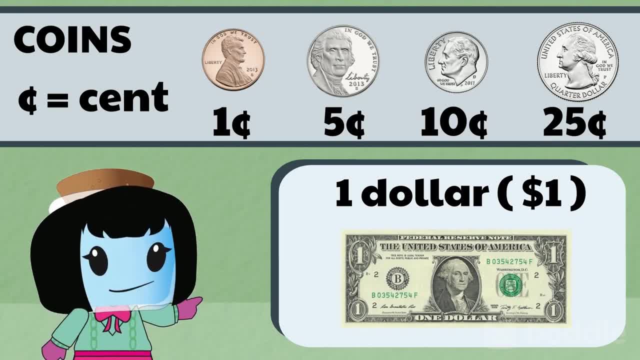 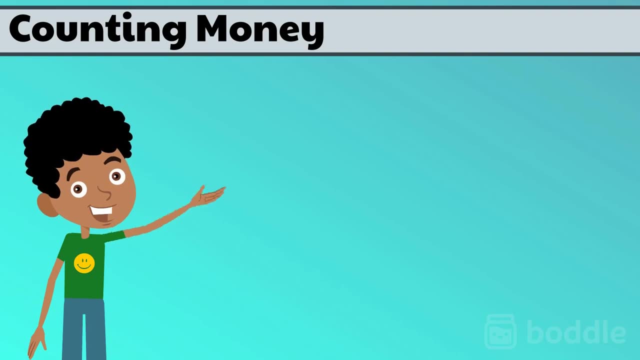 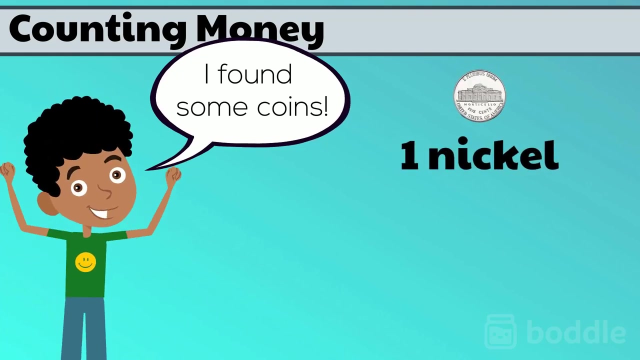 though we have a one dollar bill. Notice how this time the dollar symbol is put here Before the number. Now that we are familiar with the coins and the dollar bill, let's practice counting money by helping our friend Edward. Edward found some coins on the ground. He found one nickel and six pennies. How much did he? 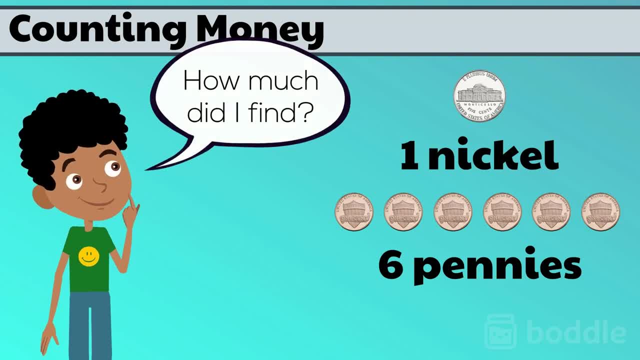 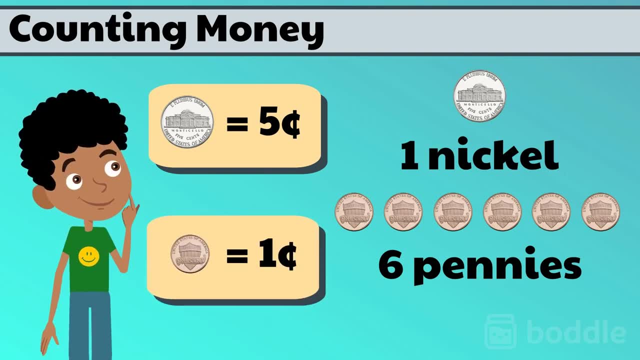 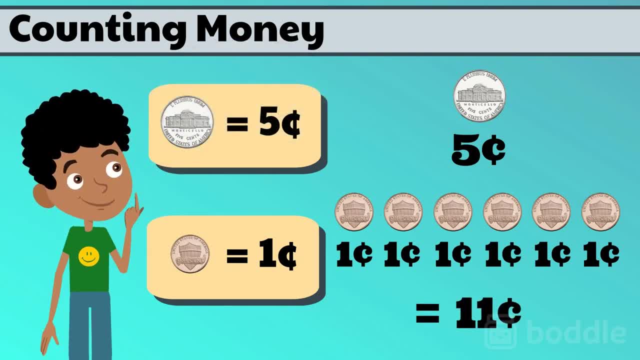 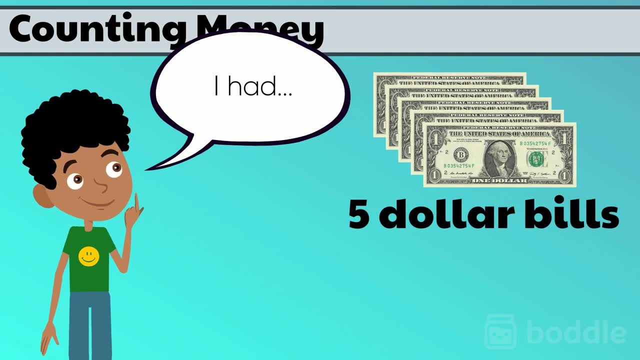 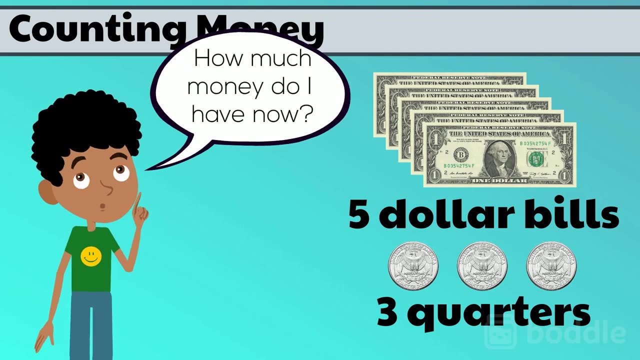 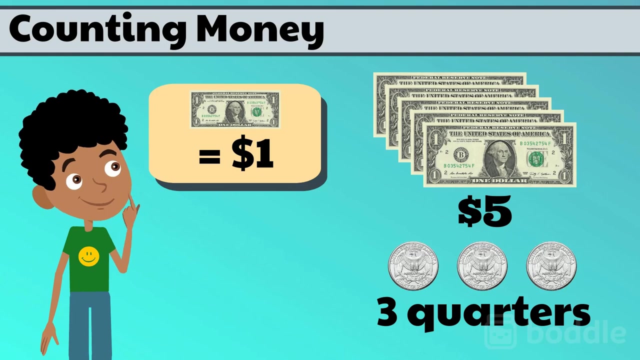 Wow, It's three quarters. However, before he found these coins, Edward already had five dollar bills and three quarters. So how much money does he have now? One dollar bill is equal to one dollar. This means five dollar bills is worth five dollars, And since Edward is, 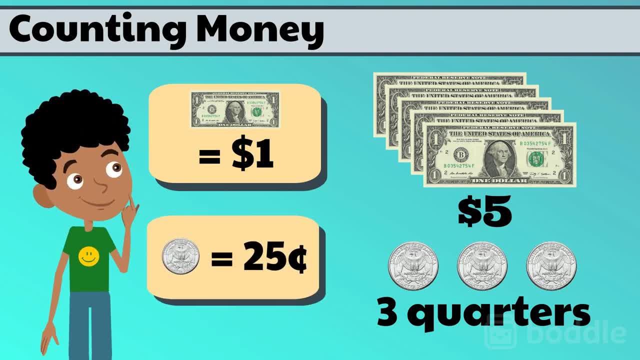 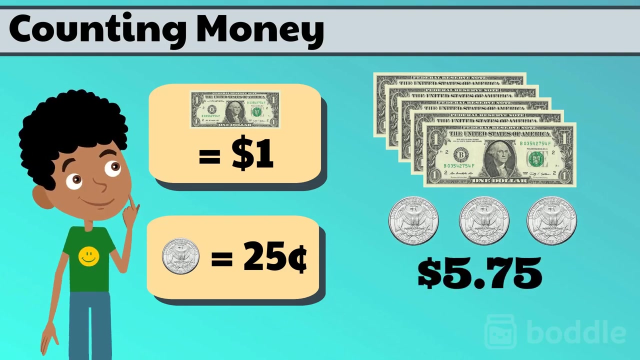 one quarter equals 25 cents. three quarters means adding 25 cents plus 25 cents plus 25 cents. so three quarters is worth 75 cents. $5 and 75 cents can be written like this: remember that Edward found 11 cents. let's add that to the. 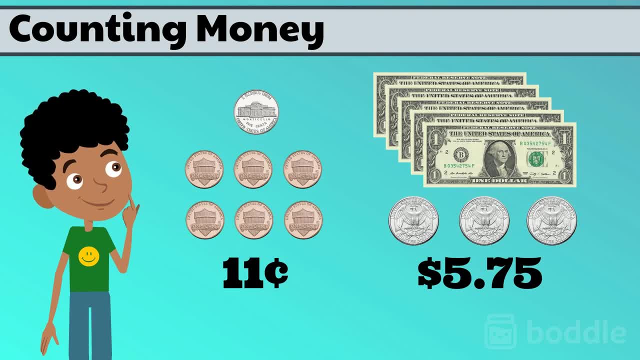 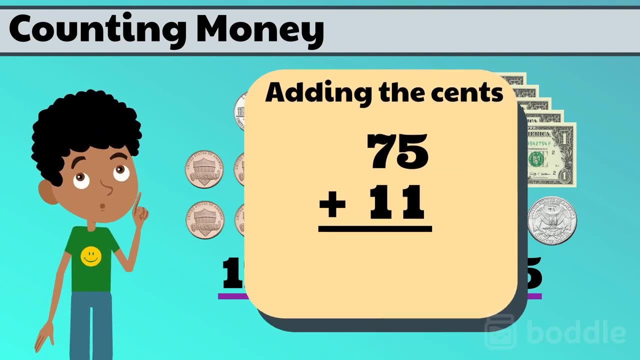 money he already had. since we're adding 11 cents, we can add it to the sense and just bring back the $5 later. let's write them again in a column and add the ones. five plus one, one equals six. adding the tens will have seven plus one equals eight, so all. 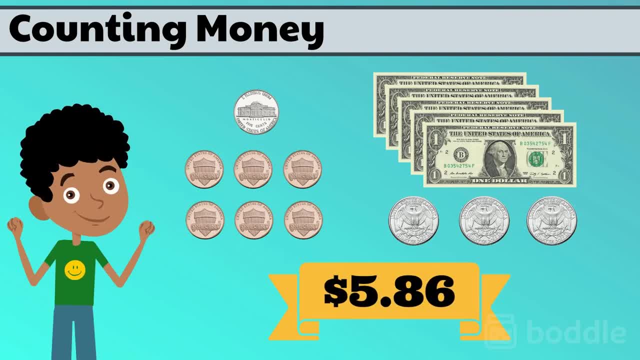 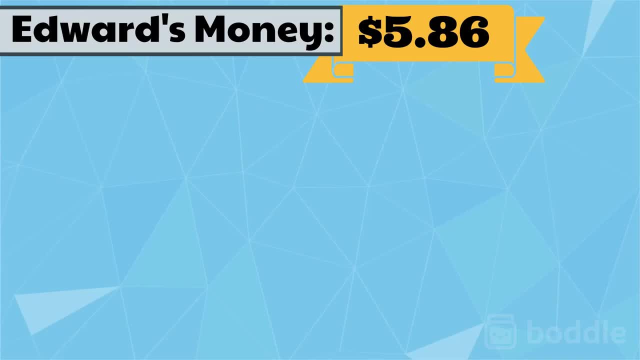 together, Edward has five dollars and 86 cents. now Edward wants to eat, so he bought some snacks with two dimes and six cents. so he bought some snacks with two dimes and six cents. so he bought some snacks with two dimes and six cents. so he bought some snacks with two dimes and 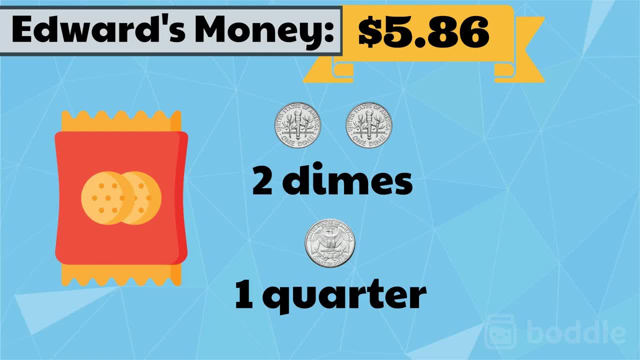 one quarter. can you figure out how much money he has left? a dime is worth 10 one quarter. can you figure out how much money he has left? a dime is worth 10 cents and a quarter is worth 25 cents. so cents and a quarter is worth 25 cents. so 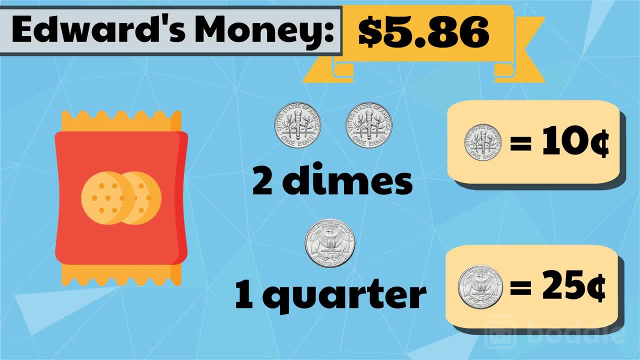 cents and a quarter is worth 25 cents. so if we have two dimes and one quarter we, if we have two dimes and one quarter we, if we have two dimes and one quarter, we need to add 10 cents plus, 10 cents plus. 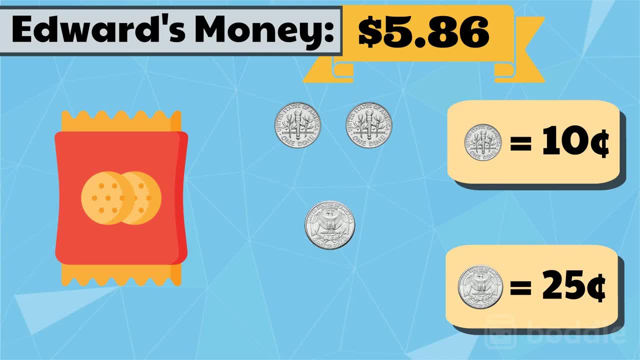 need to add 10 cents plus 10 cents. plus need to add 10 cents plus 10 cents plus 25 cents. so Edward spent 45 cents for 25 cents. so Edward spent 45 cents for 25 cents. so Edward spent 45 cents for his snacks. 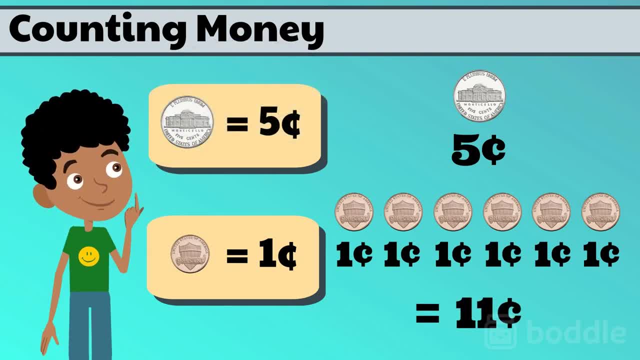 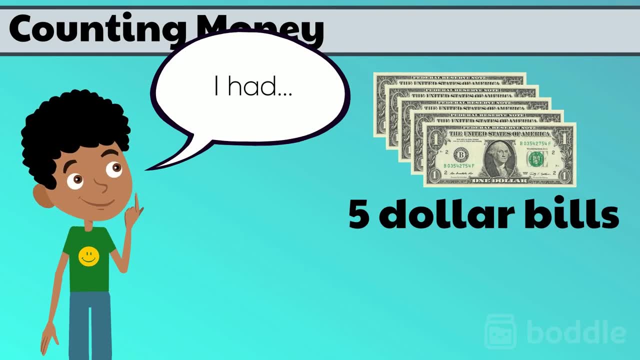 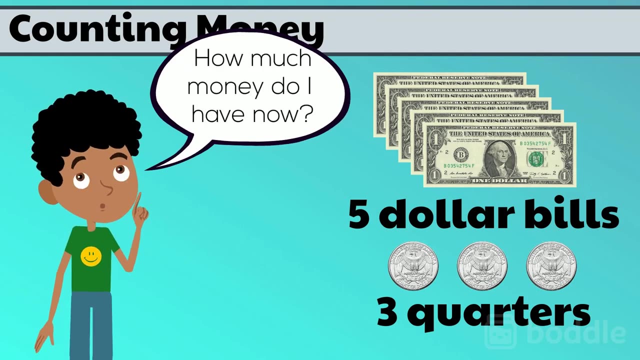 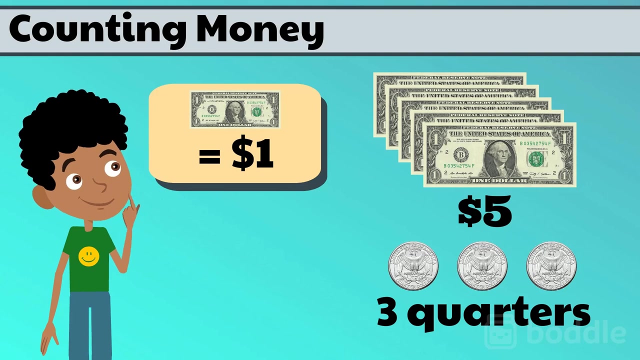 Wow, How much money. However, before he found these coins, Edward already had five dollar bills and three quarters. So how much money does he have now? One dollar bill is equal to one dollar. This means five dollar bills is worth five dollars And since one quarter equals twenty-five cents, three quarters means adding twenty-five cents. 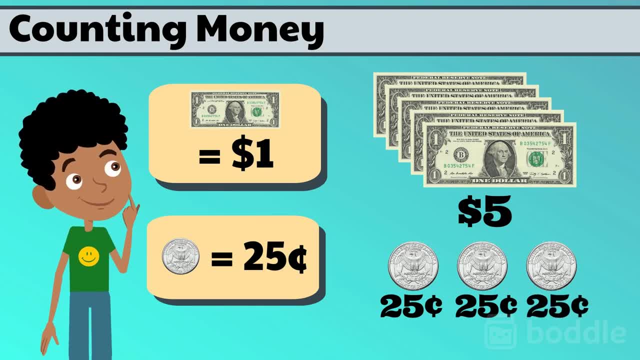 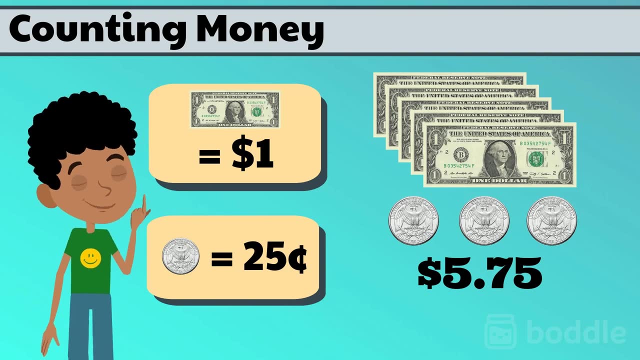 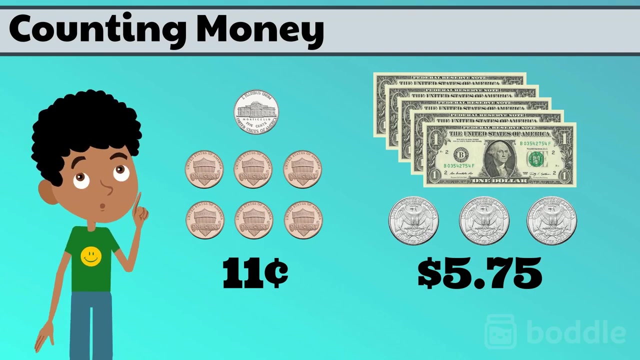 plus twenty-five cents plus twenty-five cents, So three quarters is worth seventy-five cents. Five dollars and seventy-five cents can be written like this: Remember that Edward found eleven cents. Let's add that to the money he already had. Since we're adding eleven cents, we can add it to the cents and just bring back the five. 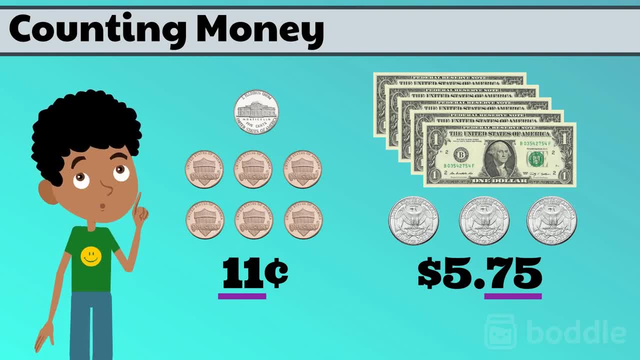 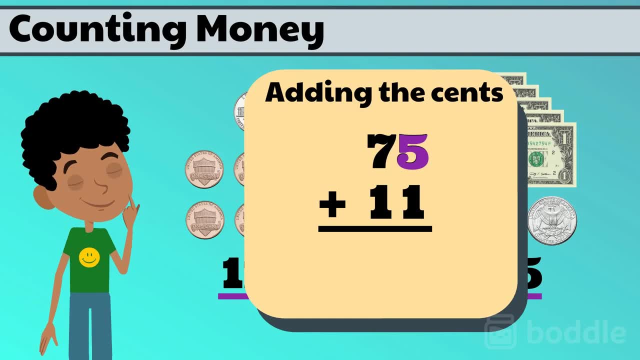 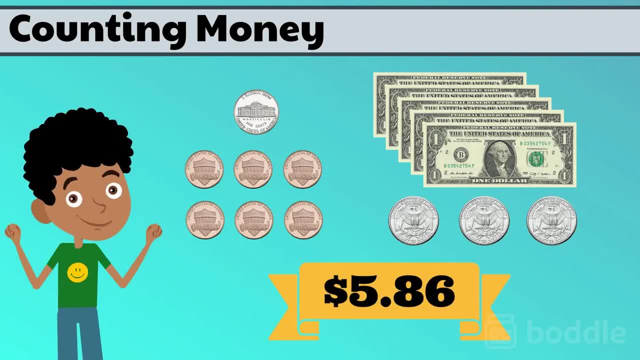 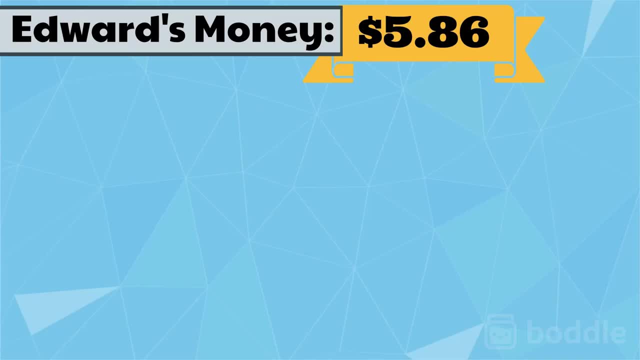 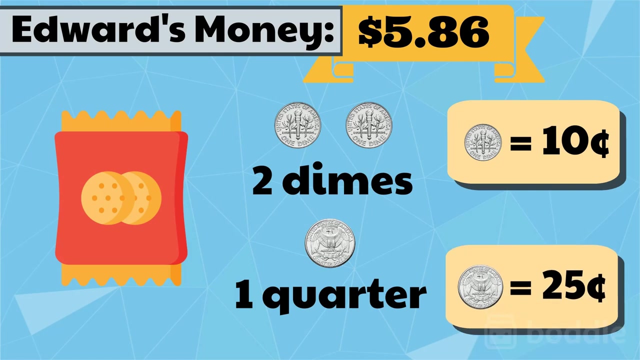 So altogether Edward has five dollars and eighty-six cents. Now Edward wants to eat, so he bought some snacks with two dimes and one quarter. Can you figure out how much money he needs? A dime is worth ten cents and a quarter is worth twenty-five cents. 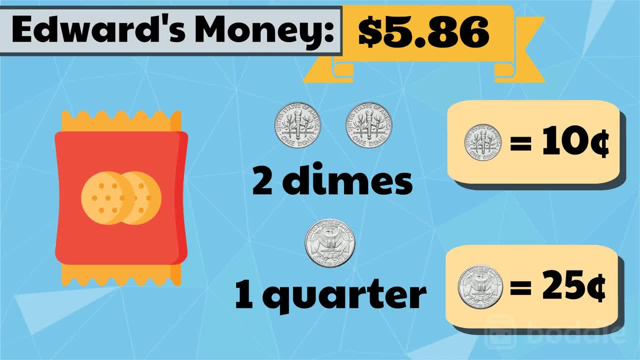 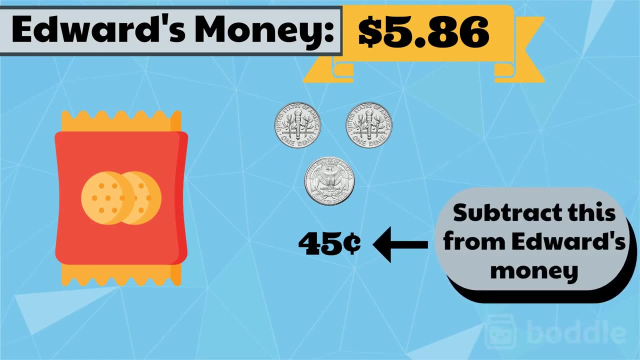 So if we have two dimes and one quarter, we need to add ten cents plus ten cents plus twenty-five cents. So Edward spent forty-five cents for his snacks. Let's subtract that from the five dollars and eighty-six cents he had. Let's subtract that from the five dollars and eighty-six cents he had. 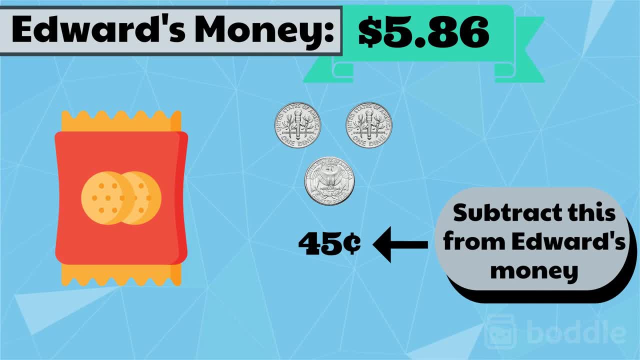 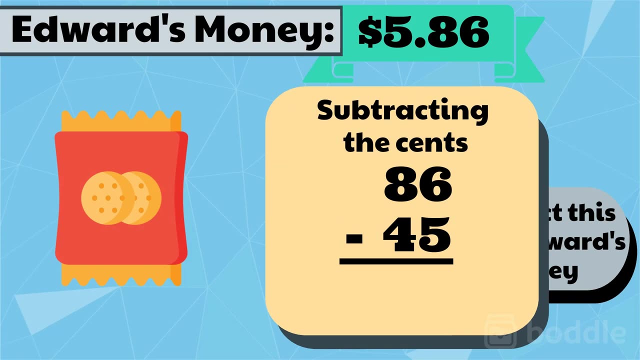 his snacks, his snacks. Let's subtract that from the $5.86 he has, Like earlier, we only have to work with the cents: 86 cents minus 45 cents. Subtracting the ones place, we'll have 6 minus 5 equals 1.. 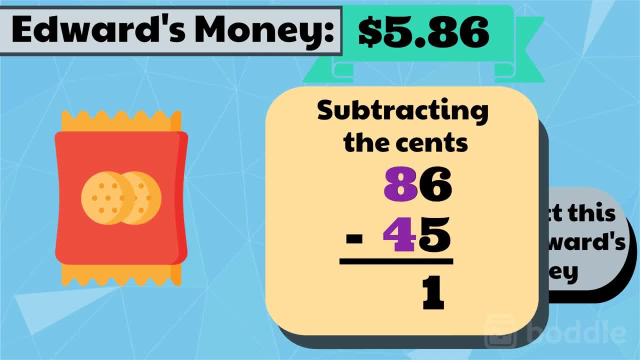 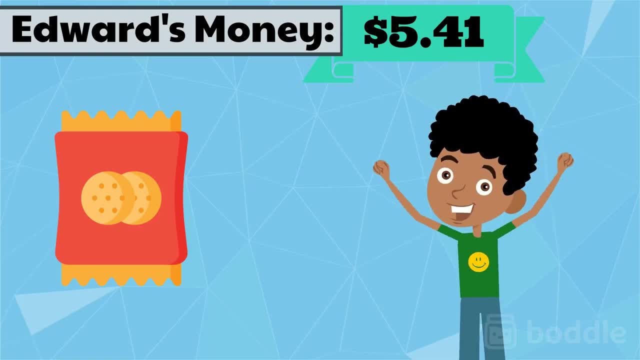 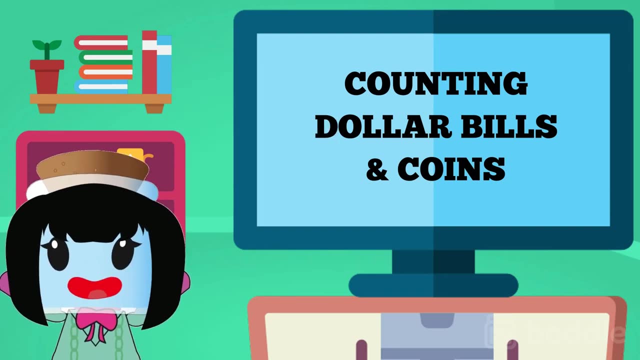 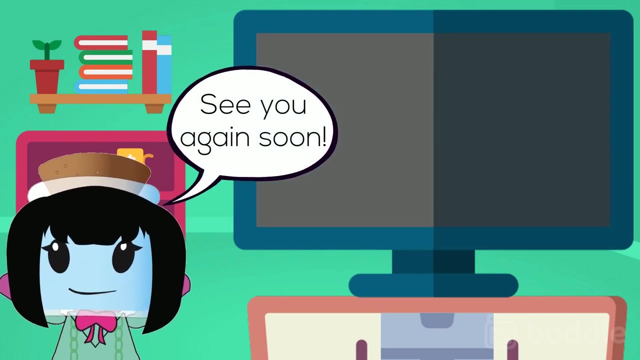 And in the tens, 8 minus 4 equals 4.. Edward is left with $5.41.. Excellent job. I hope that helped you learn more about counting $1 bills and coins. See you again soon. Are you looking for more fun ways to learn math? 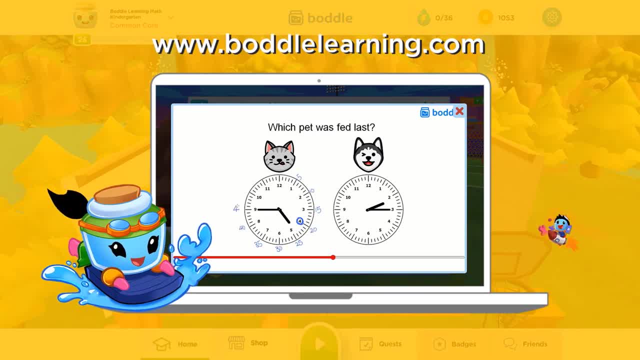 Check out Bottle Learning And access thousands of math skills all through a fun 3D game. Just visit BottleLearningcom and sign up today. 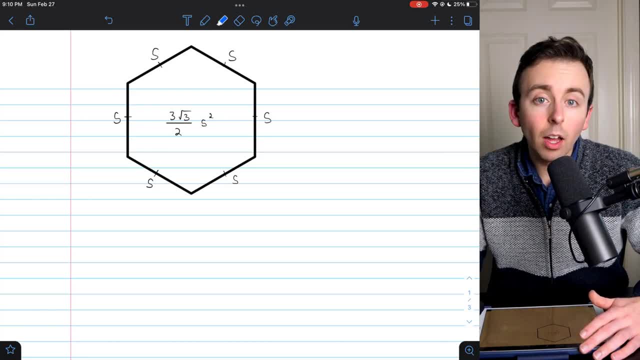 Hi, there I'm going to show you how to calculate the area of a regular hexagon. Remember, regular means that all of its sides have the same length. So in this picture we've got a regular hexagon. Hexagon has six sides, remember. 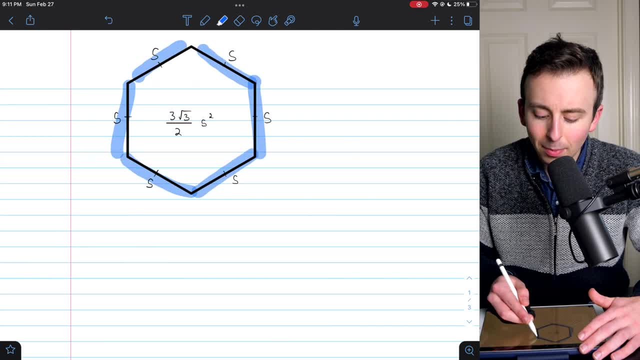 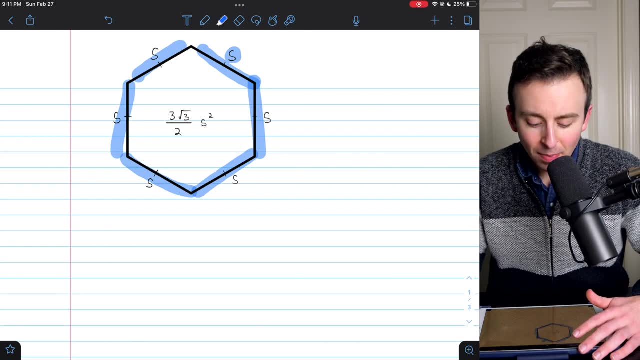 And all six sides of this regular hexagon have the same length, just a generic length that we're going to call s, And we'll look at a couple specific examples in a couple minutes. Now let's cut straight to the chase. I'll show you what the formula is. we'll do a couple examples. 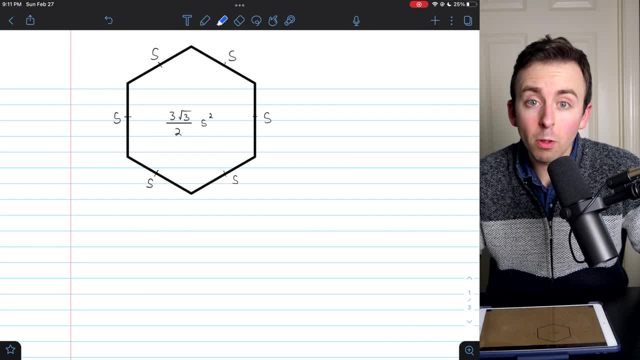 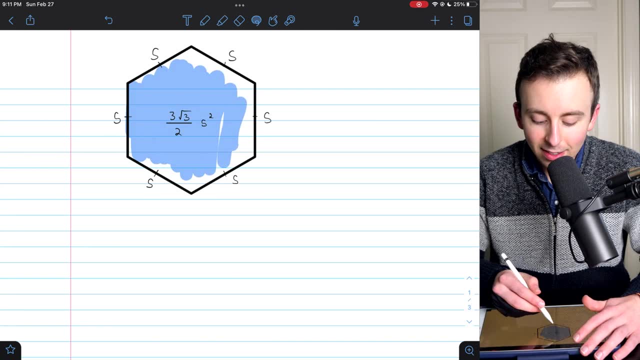 and then hang out for a couple minutes and I'll show you a little bit about where the formula comes from. The area of a regular hexagon, of course, is all of this space inside of it, And inside that space I have conveniently written the formula to calculate the area. 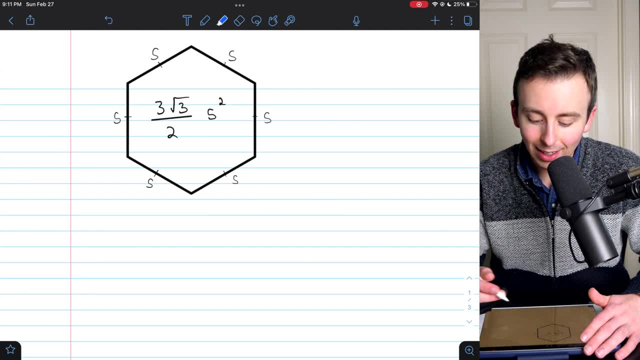 So what is the area of a hexagon whose side lengths are all s? It's just 3 halves times the square root of 3 times s squared. That's it. That's the formula. Get a regular hexagon with side length s.